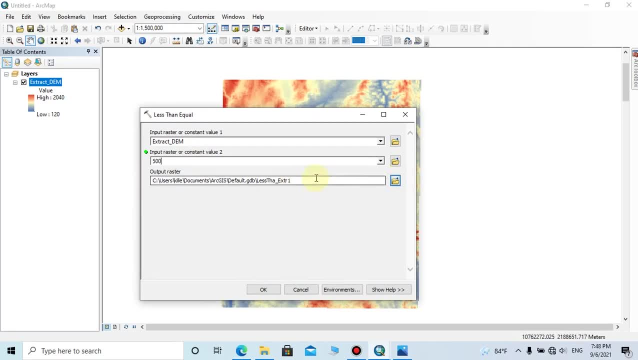 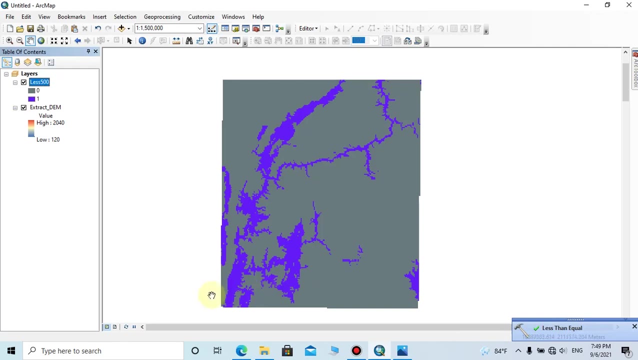 And you can change the output location and output name here. Then click on ok. Now the water level area which is equal and below 500 is formed. So the zero value part should be removed with removing color and value 1 part should be assigned suitable color. 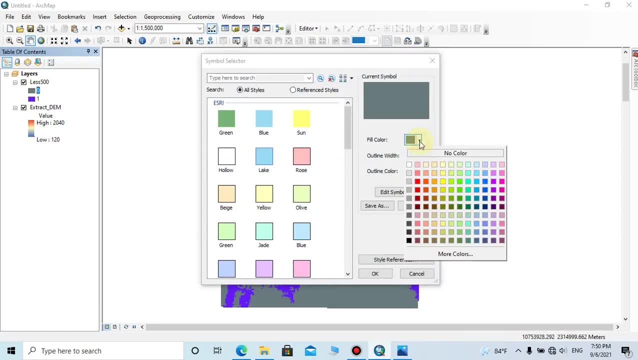 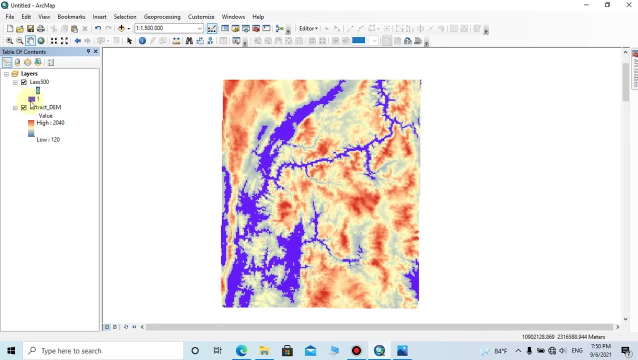 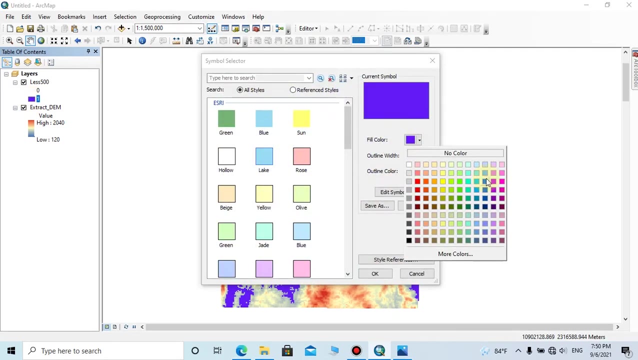 Here I am going to change the colors of zero. Here you can change the fill color as no color and outline color It's no color. Then click ok And you can assign a suitable blue range value for this one value. Here I am going to assign a light blue for this area. 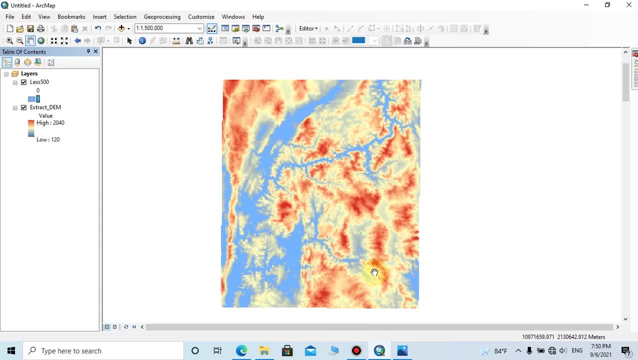 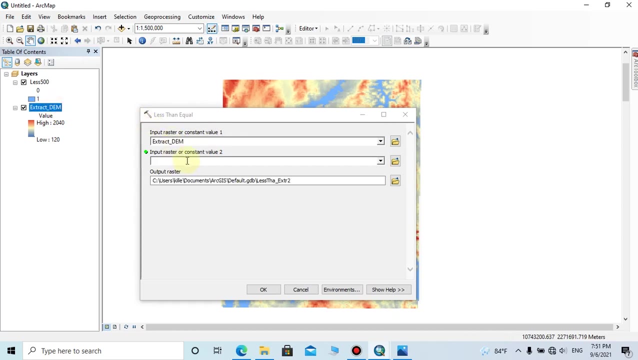 By following this method, we can extract the area which has dam value less than or equal 400.. Because this is the second flood level interval, As I mentioned earlier, The input raster value 1 should be the dam And the input raster value 2 should be typed as 400.. 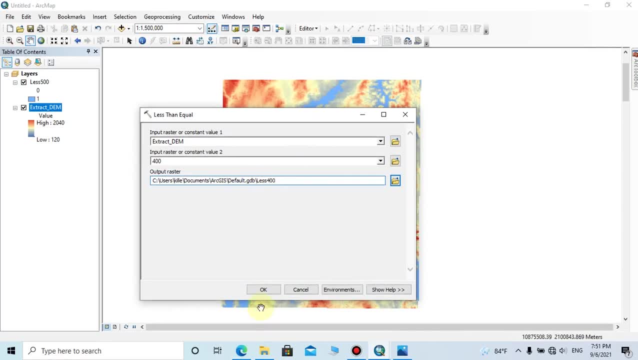 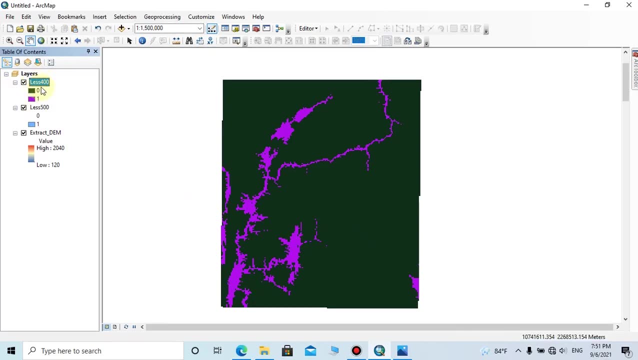 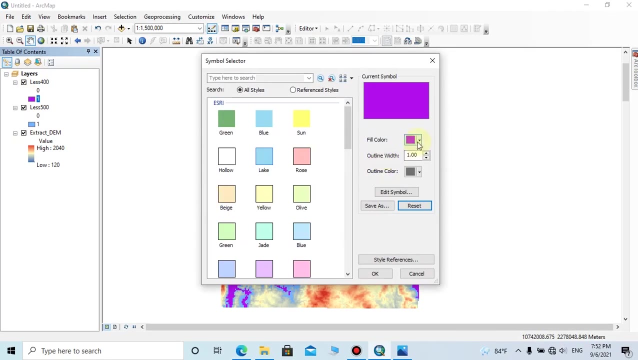 And you can change the name or location from here. Then click ok. Now the dam which has value 400 and less than 400 is formed Here. also, zero value should be removed and value 1 should be colored Here. I am going to choose a small amount of dark blue for this than the previous one. 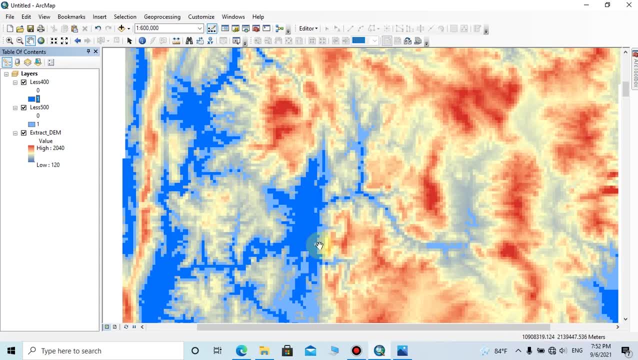 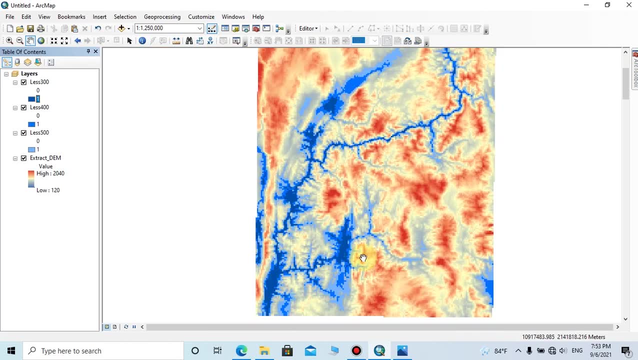 Here you can clearly see the difference of the two flood levels. By following this method, we can extract the area which has dam value less than or equal 300.. Now all the flood level have been created and colored with blue range colors. Then we should create three polygons for these three flood value areas. 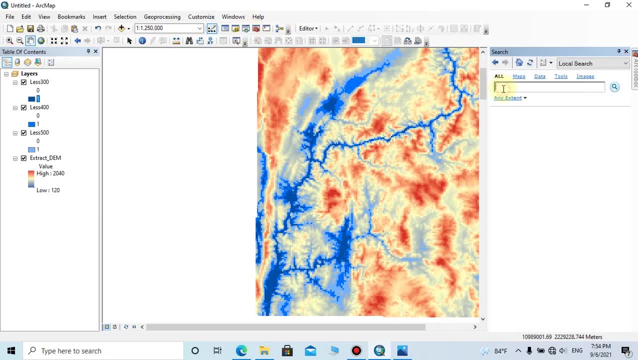 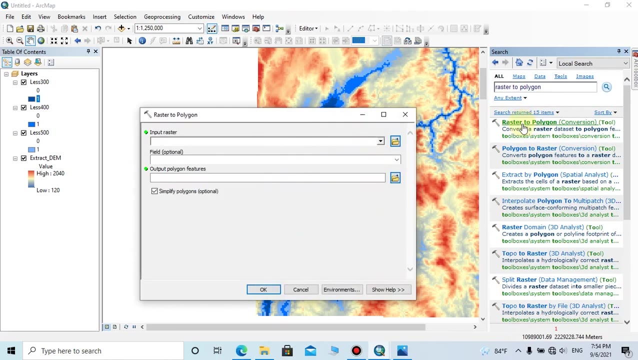 To do that, click on search tab, Then type as raster to polygon, Then click on search. Here you can choose the raster to polygon tool. Now I am going to add the input raster as 500 dam value And the field should be value. 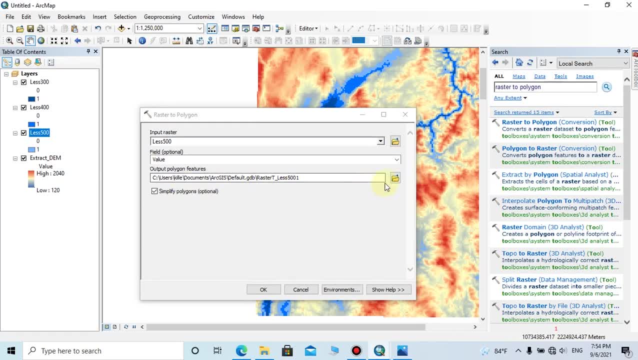 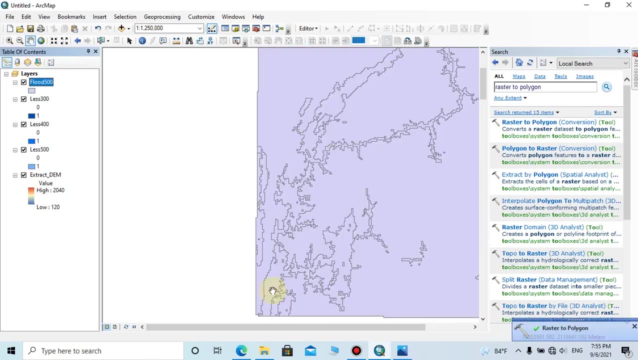 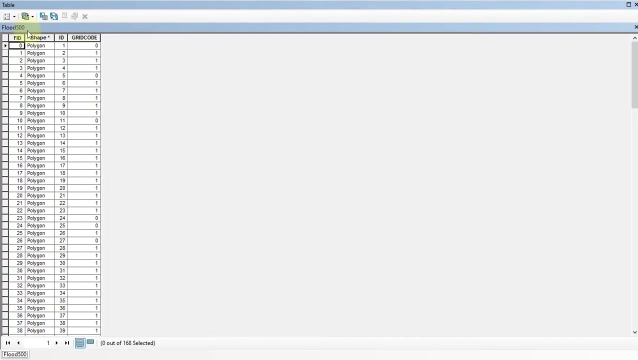 Then you can change the output location and folder name. here You should remember to tick off the tick in simplify polygon. Then click on ok. Now complete polygon has been created And by opening attribute table of this polygon You can see in grid code column there are only two values. 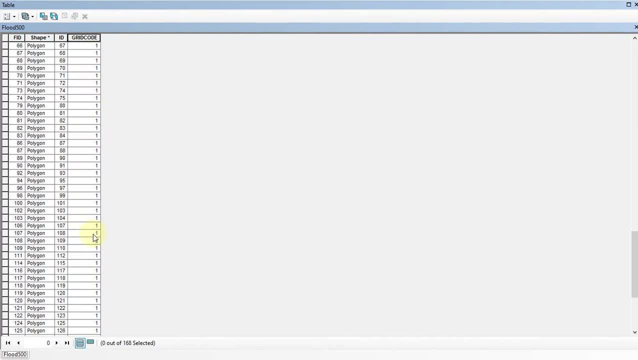 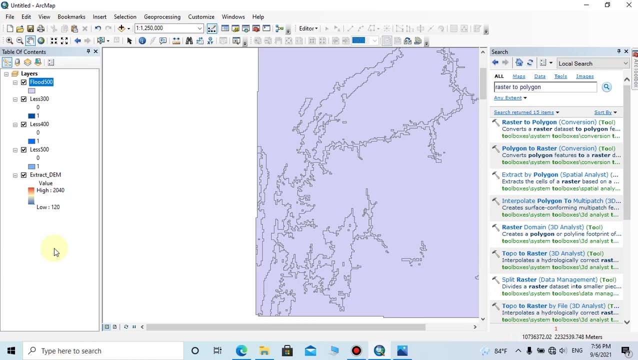 Which belongs to 0 and 1.. In here the 0 value is not included to our defined area. It means only value 1 area is the area which has maximum flood level. We need not to put these 0 value polygons So we can build in a query for this polygon. 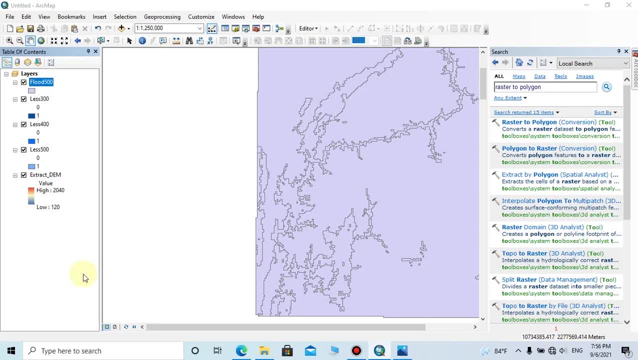 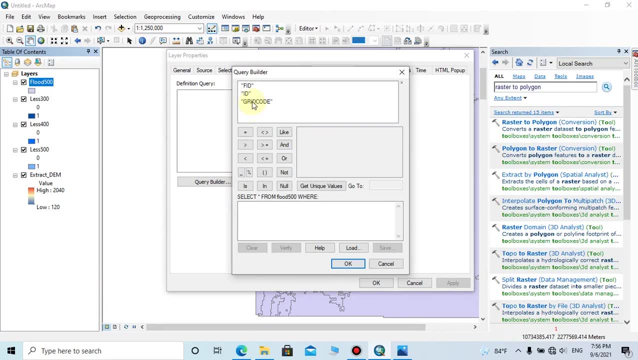 To do that, right click on this polygon and go to properties. Here you should choose define query tab. Then click on query builder. Here you should be. double click on grid code, Then click on equal, Then click on get unique values tab. Here you can see the 0 and 1 value. 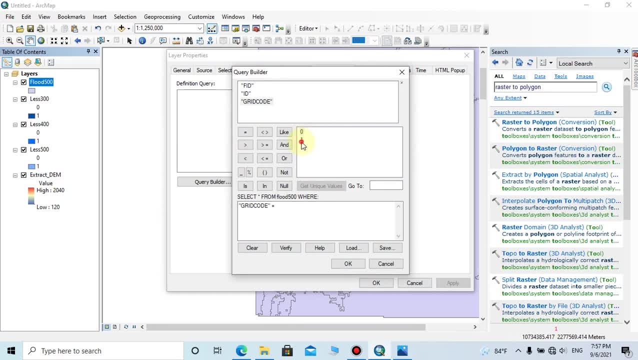 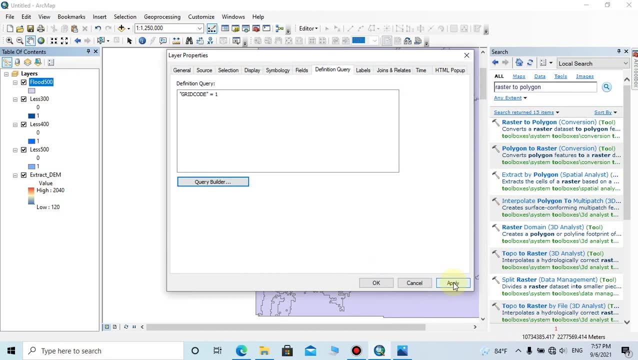 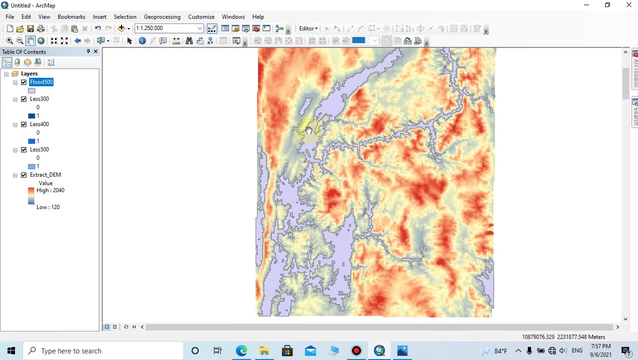 We want only one value, So we can double click on one. Before click on ok, we can verify the expression we have created, Then click ok. Then click apply. ok. It's better to change the color of this area Because it is the most damaged area in high water level. 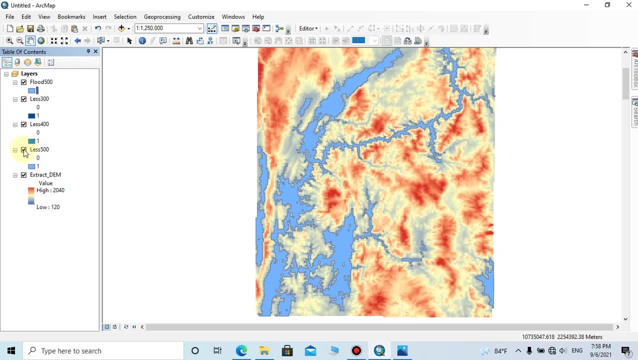 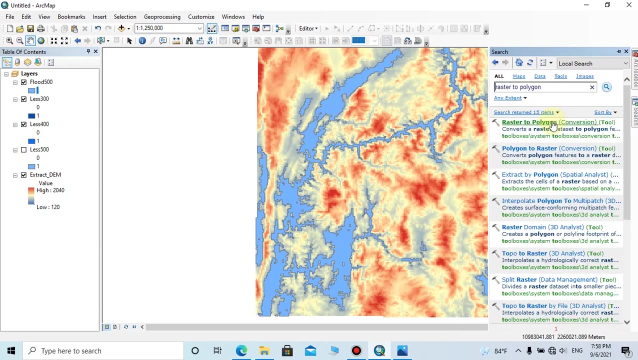 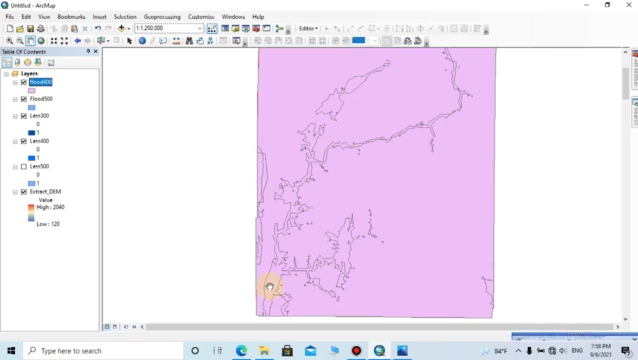 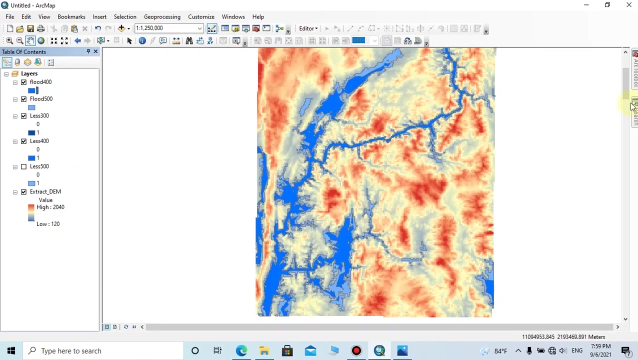 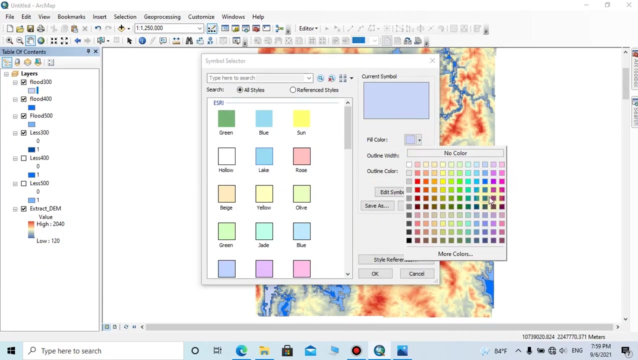 After creating this polygon, we can turn off the dem value below 500.. By following this procedure, we can create other two polygons And assign suitable colors with respect to the facade. Now we have inundation map with three water levels with different flood levels. 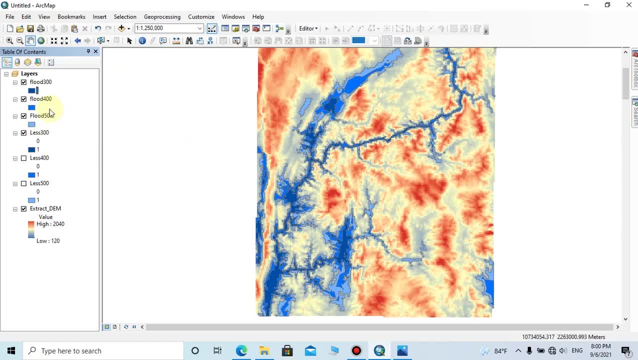 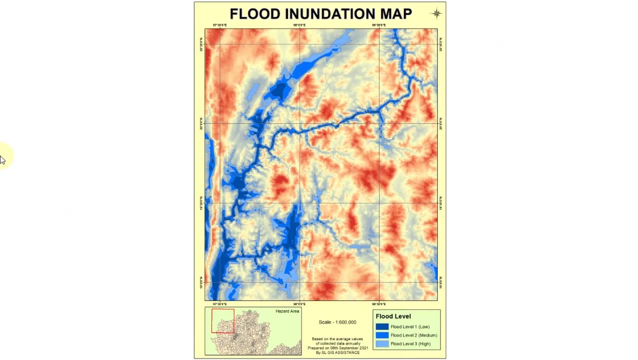 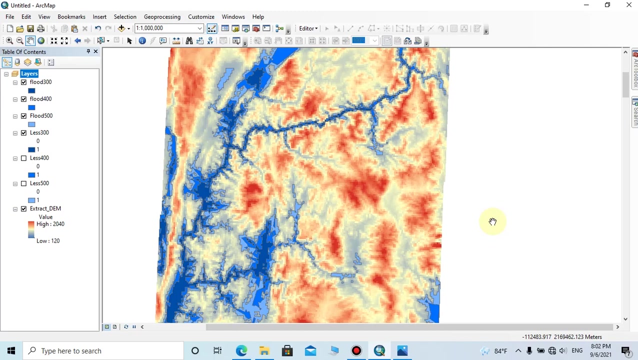 You can add marginal information for this layout and export a meaningful map. This is the map which I have prepared with the flood analysis. Here you can follow my previous lesson regarding preparing a map layout video For preparing a complete map. Let's assume you should have calculated extent of these affected area separately. 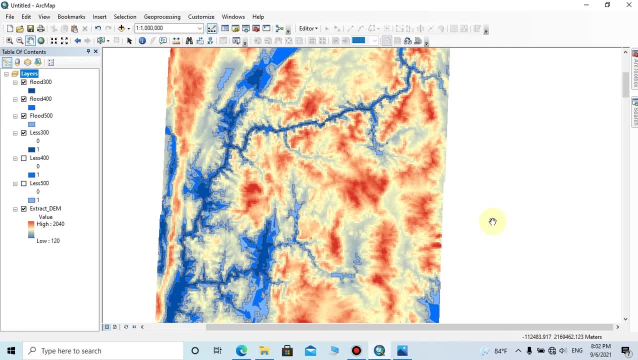 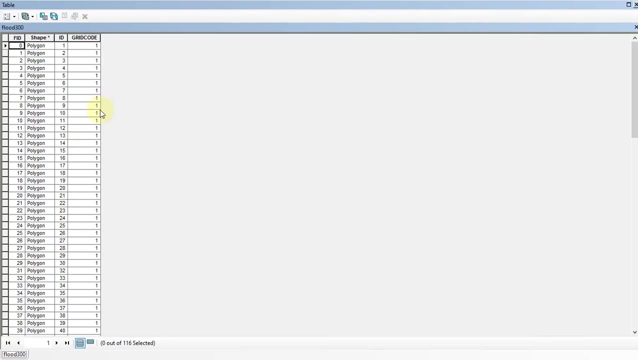 For kind of disaster management purposes. To do that we should have add new columns for extents in these every polygons. If you want to calculate low flood area, first Right click on flood 300 polygon And click on open attribute table Under this table option tab. 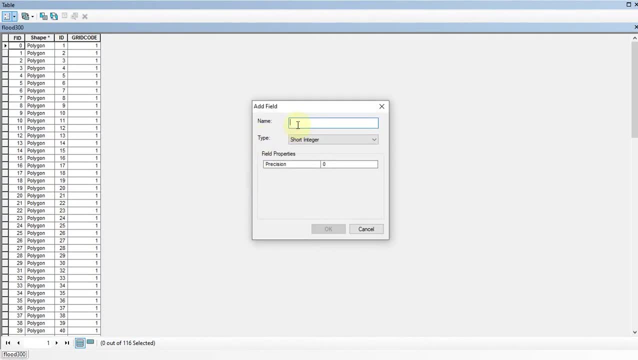 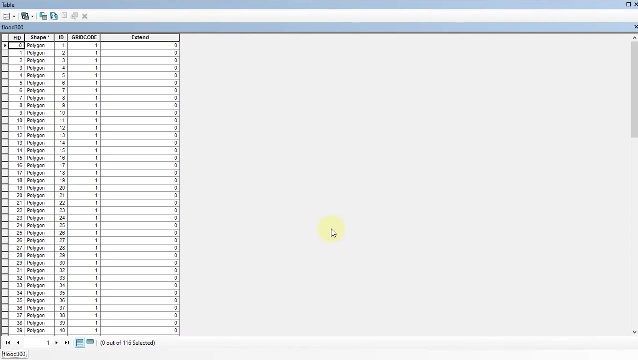 You can select add field. Here I am going to type the name as extend And change the type as double, Then click ok. Now we can calculated areas by right click on the newly added column, Then click on calculate geometry. Here the property should be select as area. 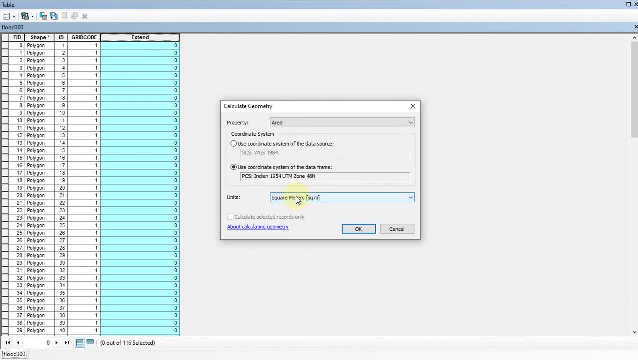 And the units can be selected as your requirement. Here I am going to select square kilometers, Then click ok. Now all the extents have been calculated And we can take the total of this column by right click on this column, Then go to statistics. 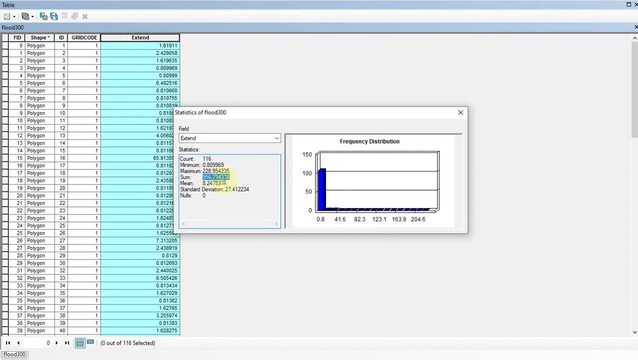 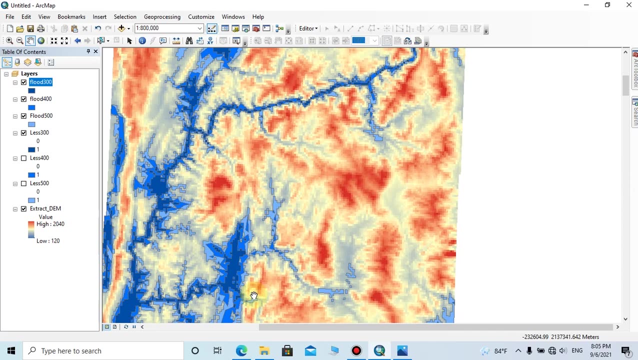 Here, the field sum display the total extent of this area. By following this procedure, We can calculate areas of these three flood level. You can take the affected area values to your project And do further analysis regarding disaster management If you want to put this inundation map to your thesis. 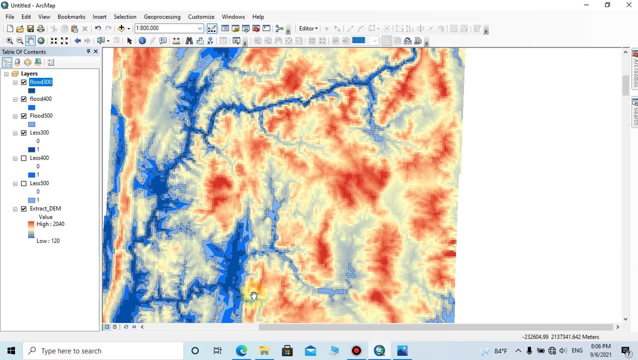 You can change these layer names And prepare quality map. Ok, this video will help you to do your further analyzing in disaster management, Such as predicting flood level in high rainfall situations And help to remove people from inundation areas. Please leave a comment regarding this video. 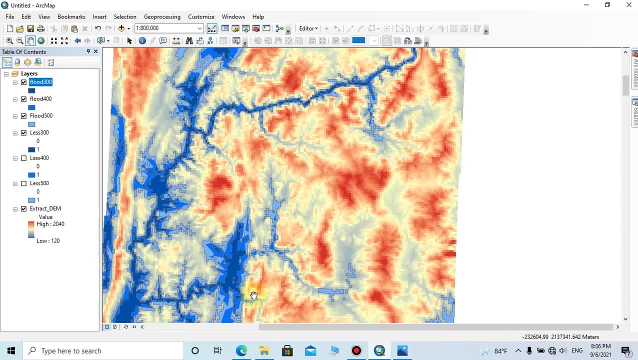 And your suggestions for next lessons. Thanks for watching And don't forget to subscribe us.